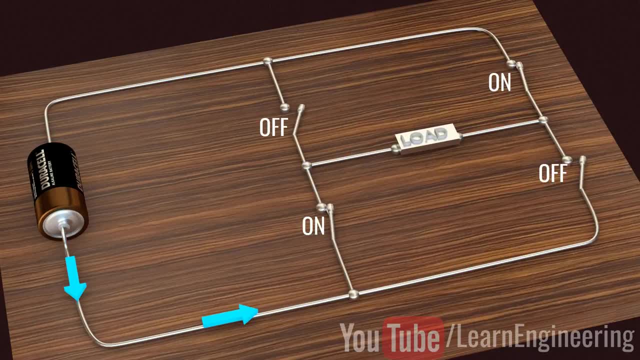 Now just do the reverse and observe the current flow. It is clear that the current flow is the opposite in this case, as is the output voltage across the load. This is the basic technique that produces a square wave alternating current. We all know that the frequency of the AC supply available in our homes is 60 Hz. 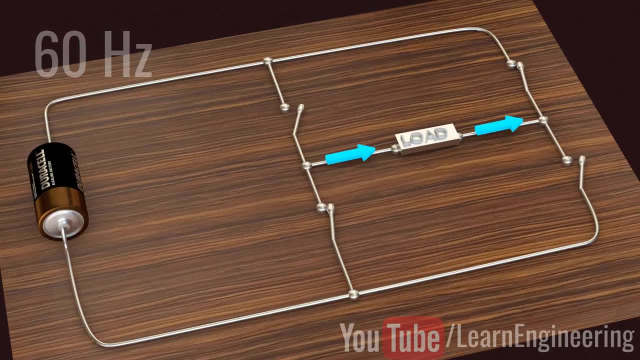 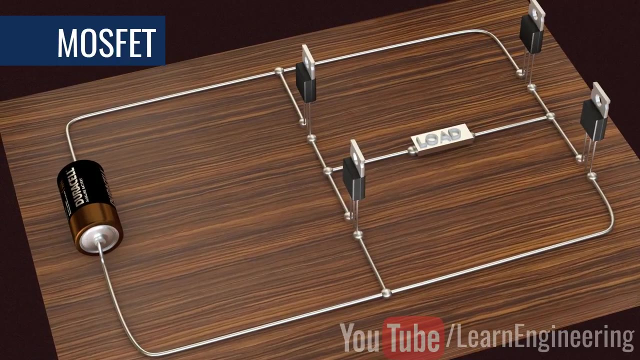 This means that we need to turn the switch on and off 120 times in a second, which is not possible, whether manually or by using mechanical switches. We introduce semiconductor switches such as MOSFET for this purpose. They can turn on and turn off thousands of times per second. 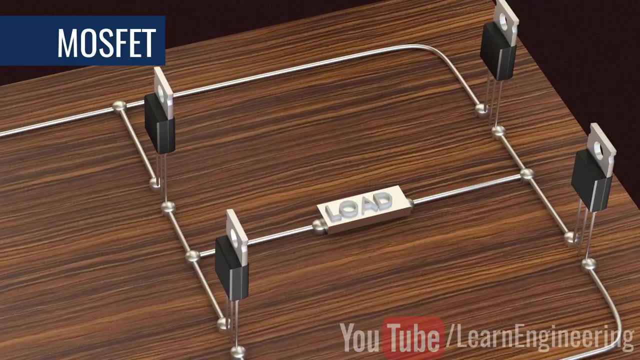 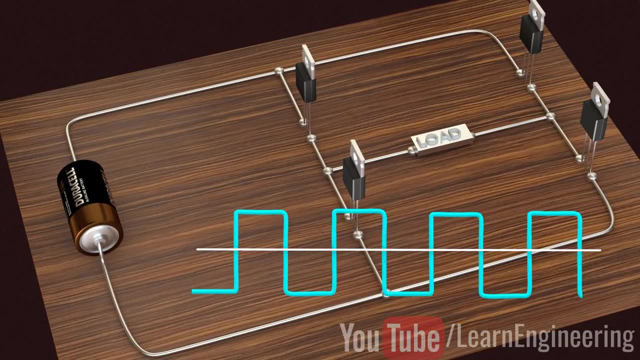 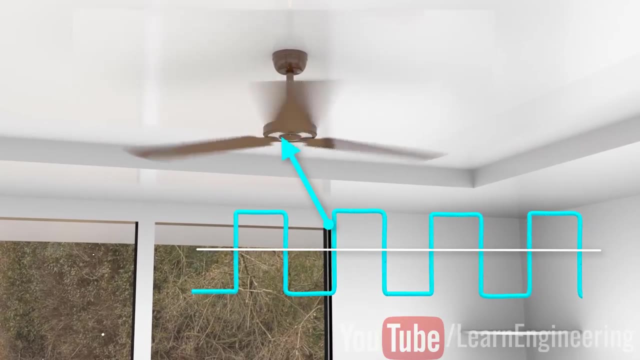 With the help of control signals, we can turn transistors on or off very easily. The square wave output is a high approximation of sine wave output. Old inverters used to produce them. That's why you hear a humming noise when you run your electric fan or other appliances using square wave power. 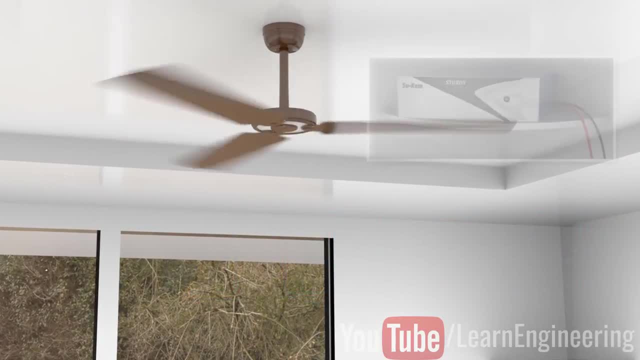 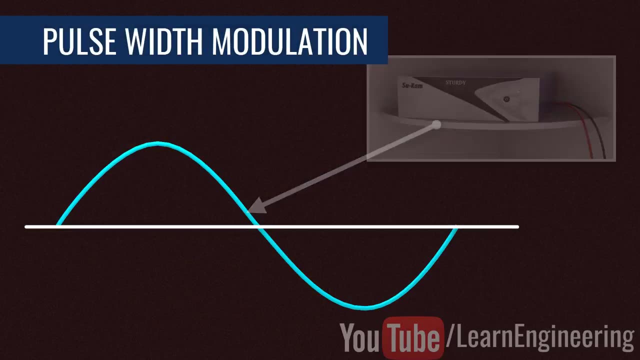 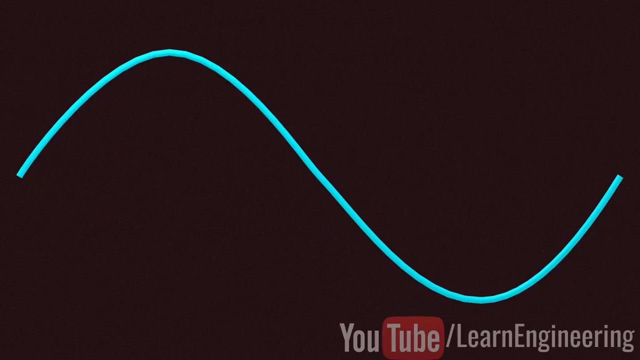 They also heat up electric equipment. Modern inverters produce pure sinusoidal output. Let's see how they achieve it. A technique called pulse width modulation is used for this purpose. The logic of pulse width modulation is simple: Generate the DC voltage in the form of pulses of different widths. 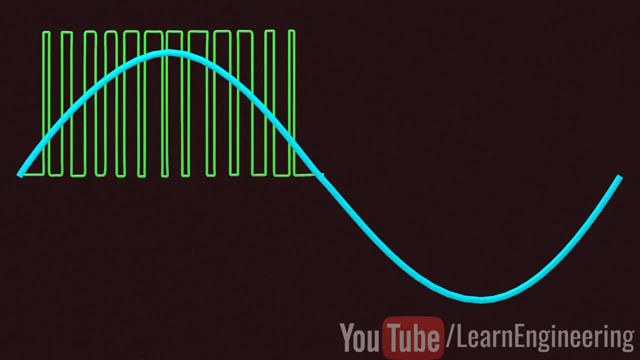 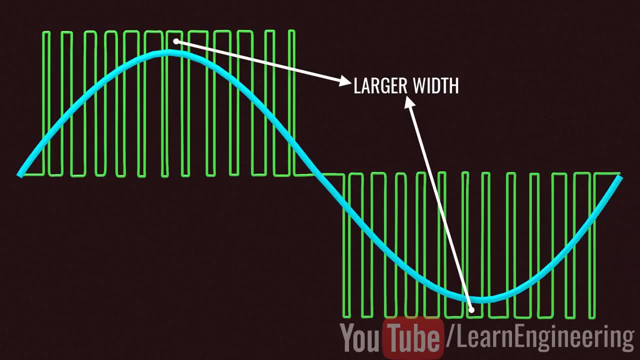 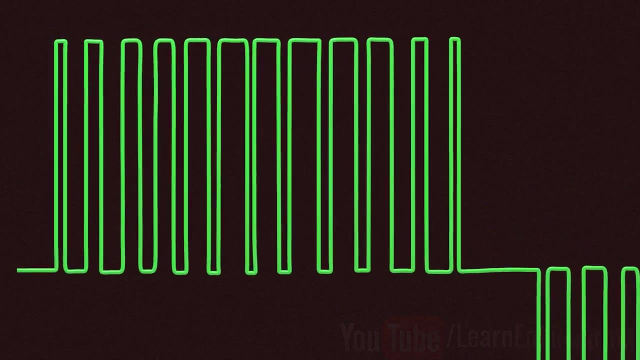 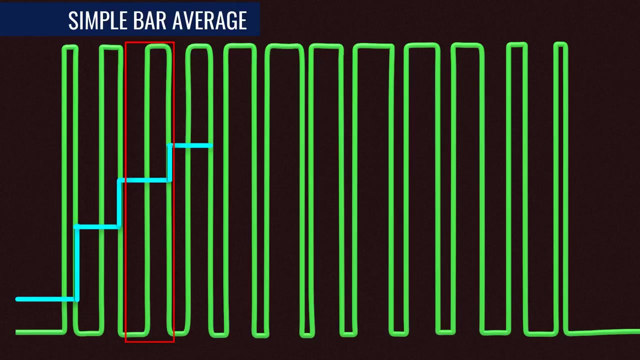 In regions where you need higher amplitudes, it will generate pulses of larger width. The pulses for the sine wave look like this. Now here is the tricky part: What will happen if you average these pulses in a small time interval? You will be surprised to see that the shape of the averaged pulses looks very similar to the sine curve. 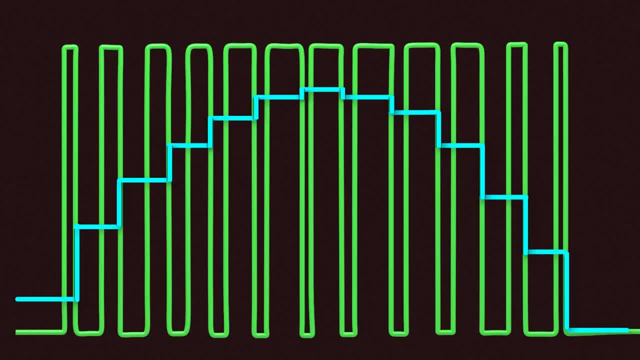 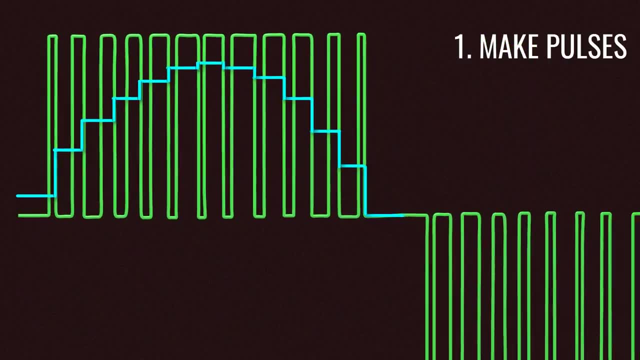 The finer the pulse is used, the better shape the sine curve will be. Now the real question is how to make these pulses and how do we average them in a practical way. Let's see how they are implemented in an actual inverter. 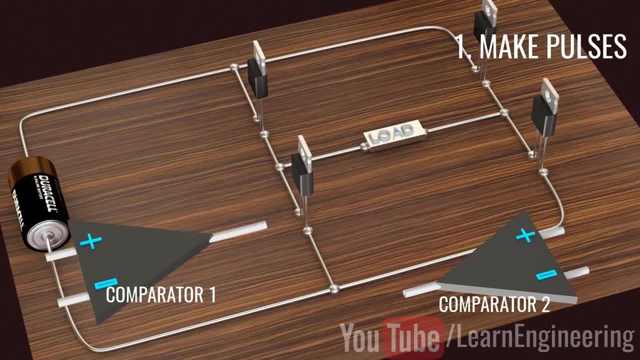 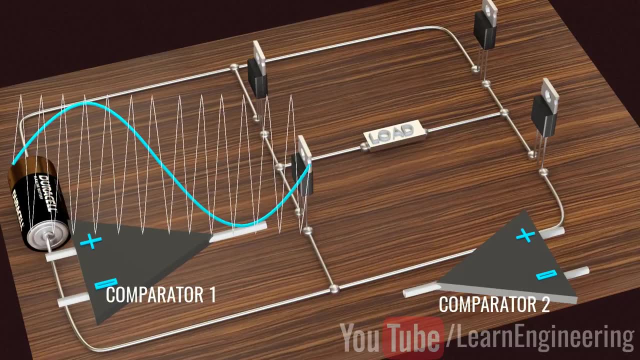 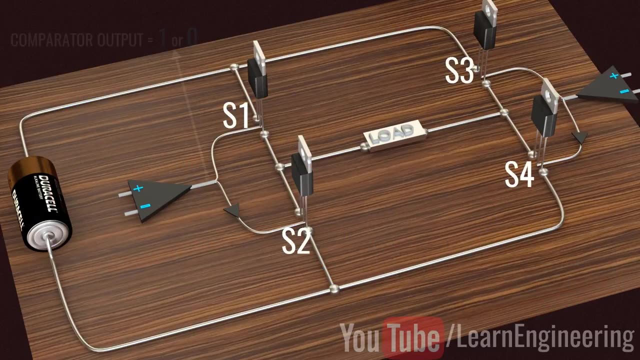 Two comparators are used for this purpose. Comparators compare a sine wave with triangular waves. One comparator uses a normal sine wave and the other comparator uses an inverted sine wave. The first comparator controls S1 and S2 switches and the second comparator controls S3 and S4. 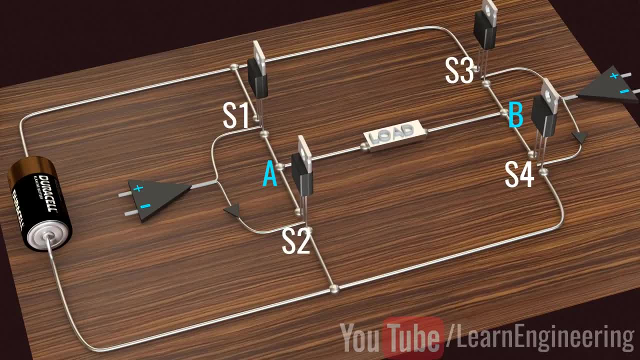 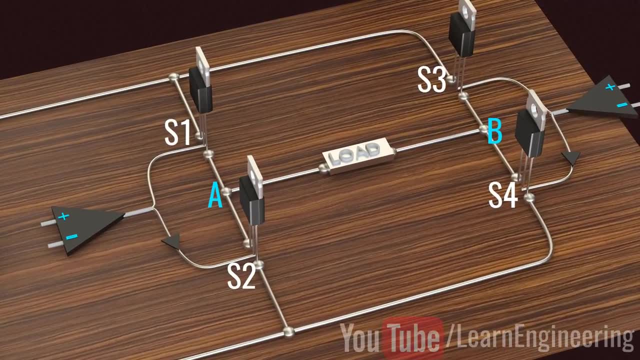 S1 and S2 switches determine voltage levels. S1 and S3 switches determine voltage level at point A and the other two switches determine voltage level at point B. You can see that the one branch of comparator output is fitted with a logic, NOT gate. 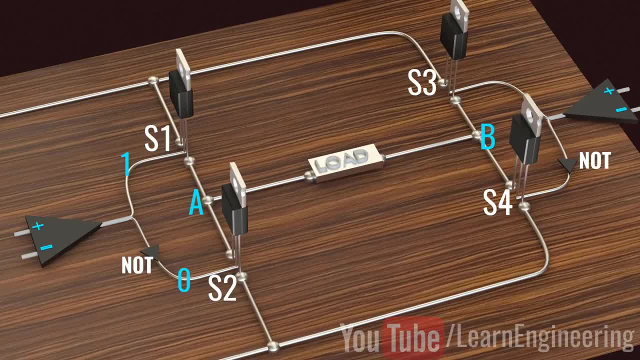 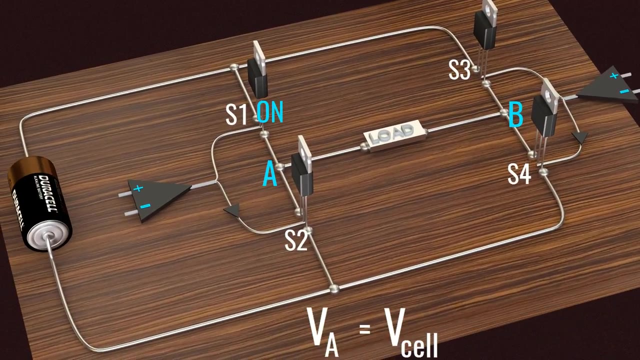 This will make sure that when S1 is on, S2 will be off, and vice versa. This also means that we can never turn on S1 and S2 at the same time, which will cause the DC circuit to short circuit. Turning S1 gives cell voltage at point A. 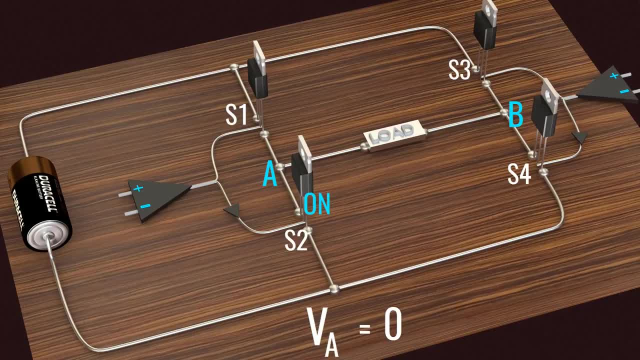 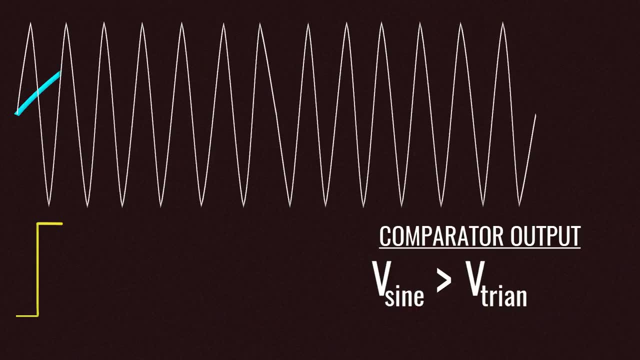 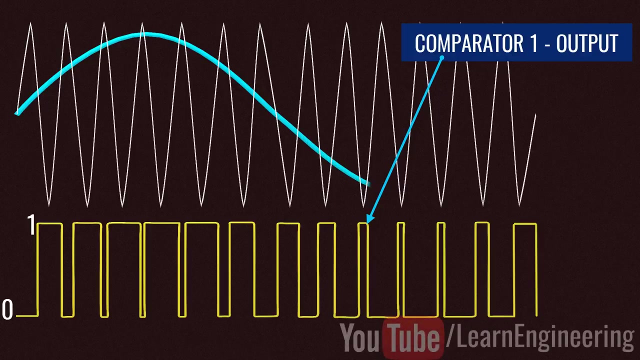 and turning on S2 gives zero voltage at the same point. Same is the case for point B. The switching logic of PWM is simple. When the sine wave value is more than the triangular wave, comparator produces one signal, otherwise zero signal. Now observe voltage variation at first comparator. according to this logic, 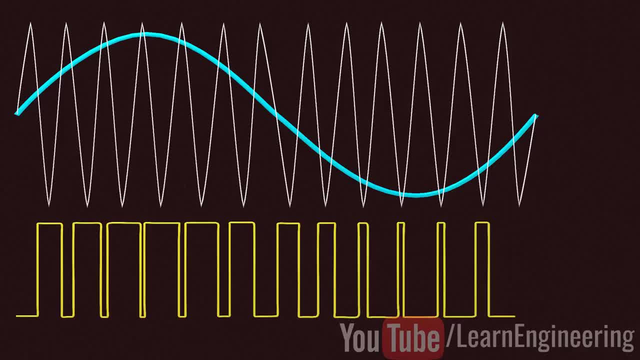 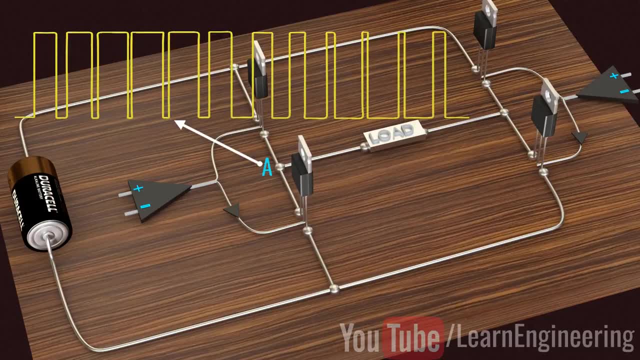 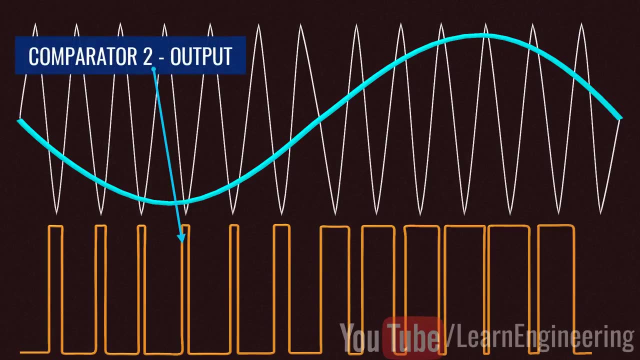 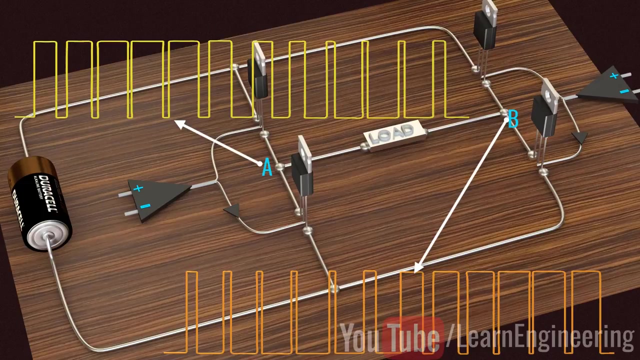 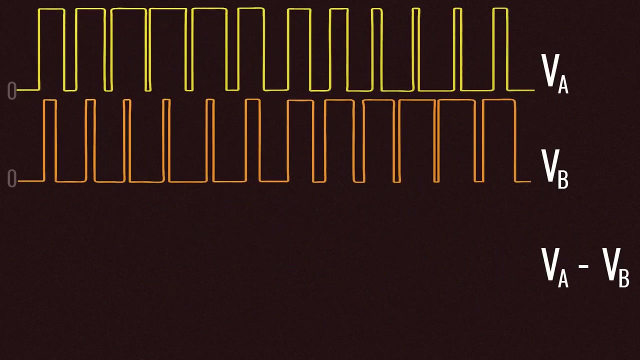 Control signal of 1 turns on the MOSFET, The voltage pulses produced at point A are shown. Apply the same switching logic and observe the voltage pulses generated at point B. Since we are drawing output voltage between point A and B, the net voltage will be the difference between A and B. 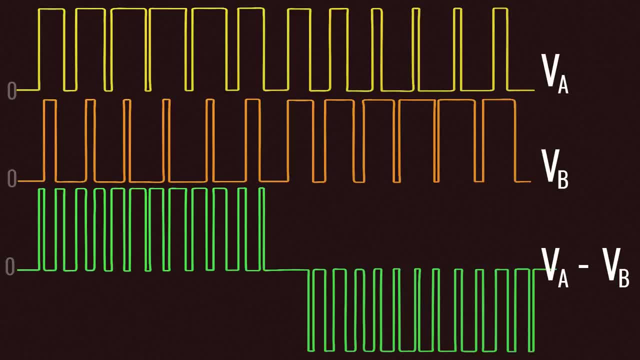 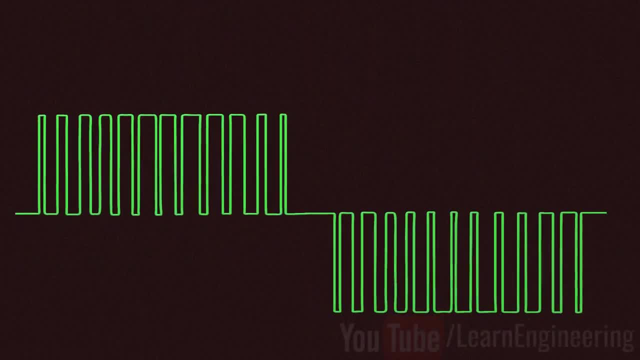 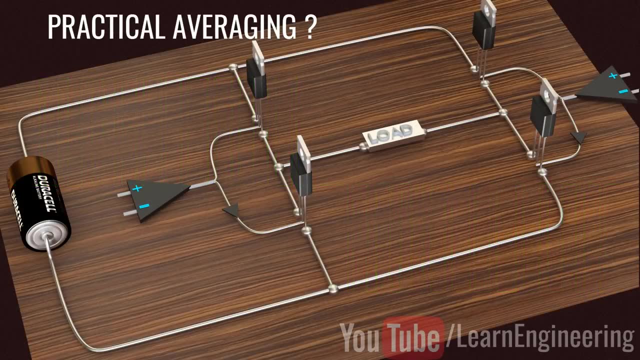 This is the exact pulse train. we need to create the sine wave. The finer the triangular wave, the more accurate the pulse train will be. Now the next question is: how do we practically implement the averaging? To make it exactly, sinusoidal energy storage elements such as inductors and capacitors. 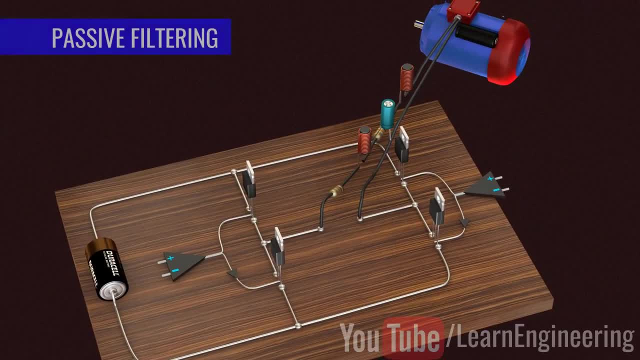 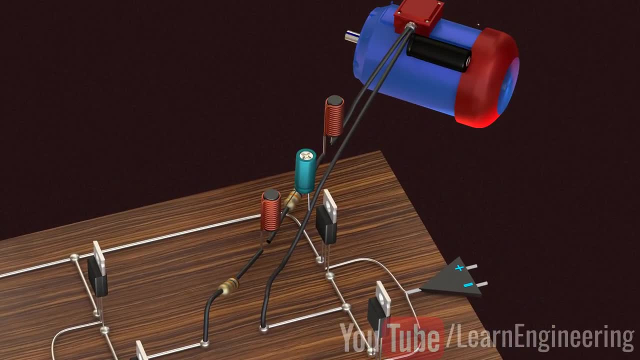 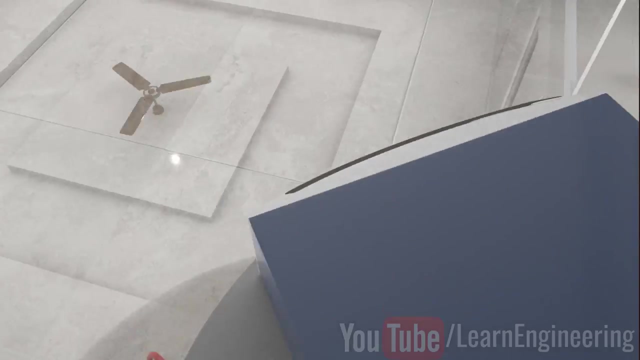 are used to smooth the power flow. They are called passive filters. Inductors are used to smoothen the current and capacitors are used to smoothen the voltage. All in all, with an inverter bridge, a good PWM technique and a passive filter. 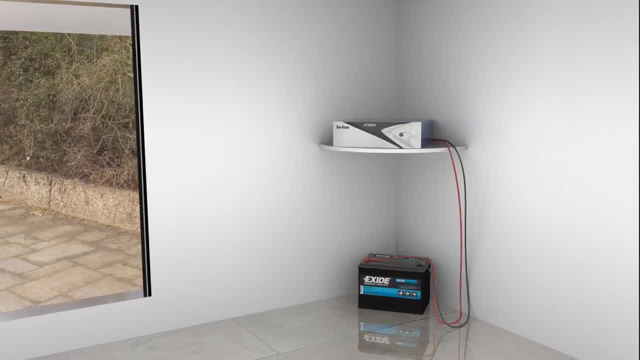 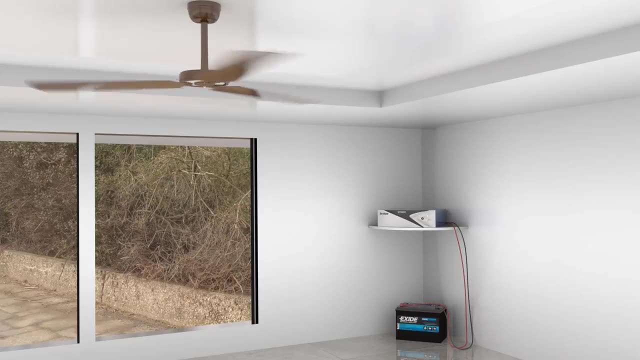 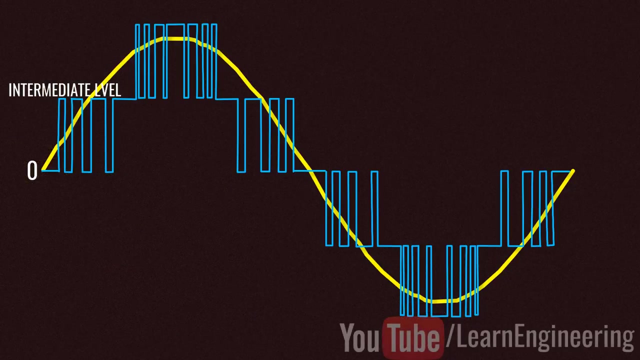 you can generate sinusoidal voltage and operate all of your appliances without any fuss. The inverter technology we have explained so far has only two levels of voltage. What if we introduce one more voltage level? This will give better approximation of the sine wave and can reduce instantaneous error.